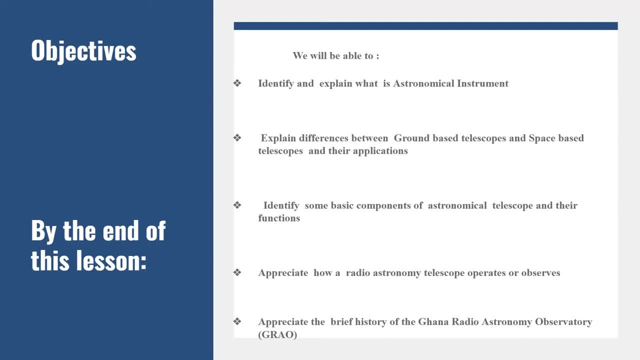 We will also find out what is an astronomical instrument. The shown effects of astronomical measurements are convenient for snowballing, нов疆hming and implied objects. In our common conflict discussion we will discuss distance multiplication and how spatial optimization can improveiamoce. the inspiration of tau and tel мер. what are the morphological expectations of the dado convention and know-it-all, and how Icelanders and the回u of history will improve their understanding of the geographic bestimmtual phenomena around this landscape? We have already spoken about the historical character of gouvernement. 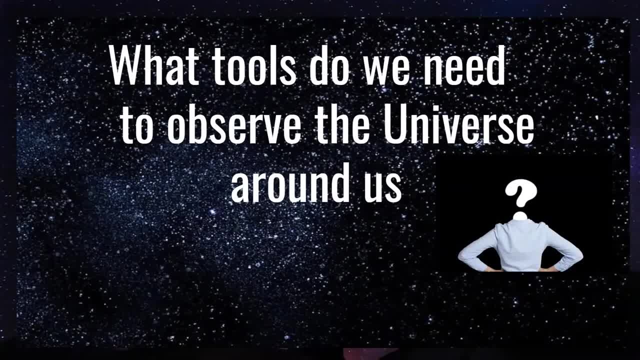 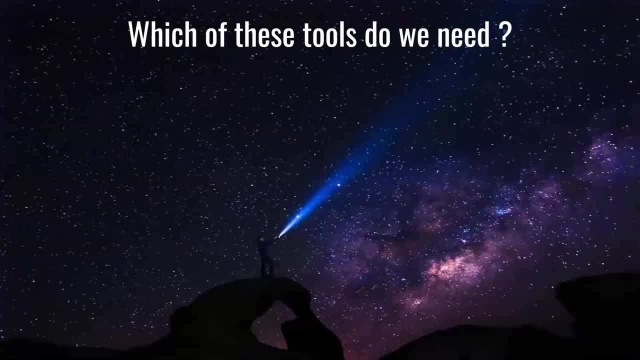 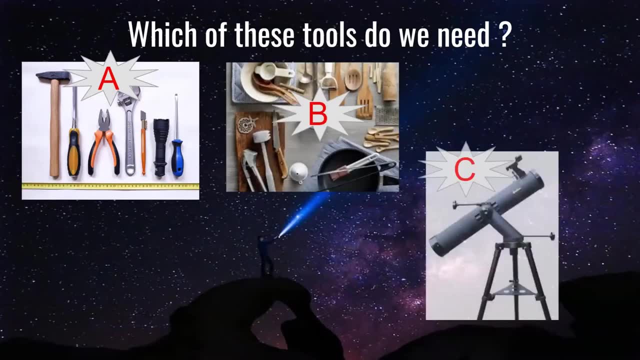 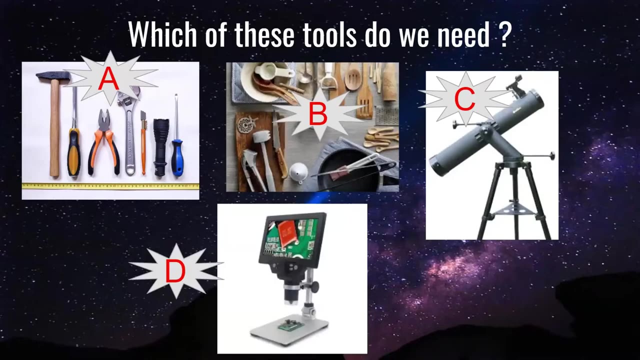 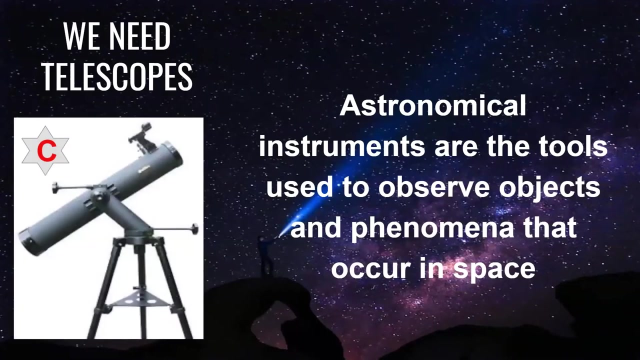 us. what is your guess? okay, so which of the following tools do we need to observe the universe? is the answer a or b, c or d? which of them? if you get it right, well done, the answer is c. now, astronomical instruments are the tools used to observe objects and phenomena that occur in 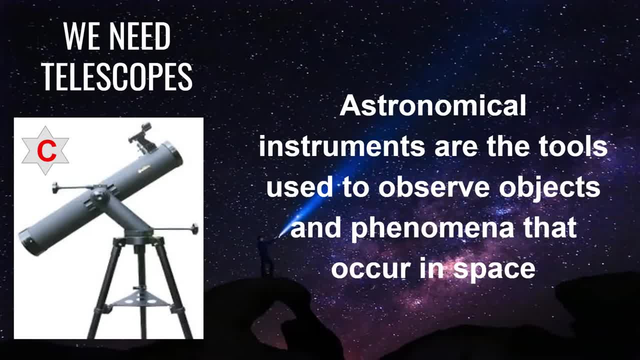 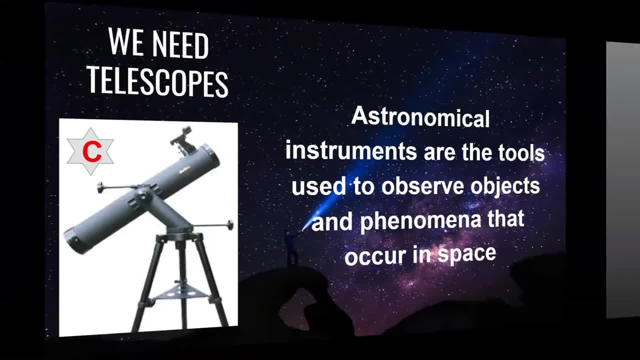 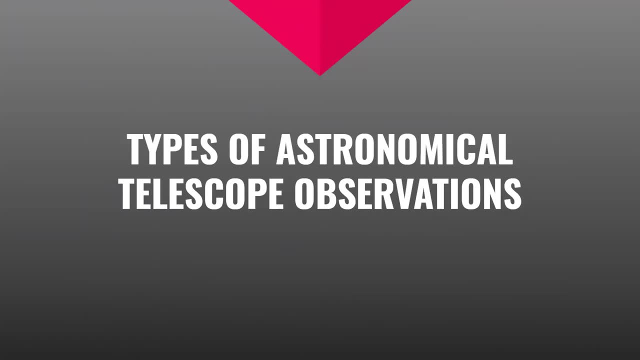 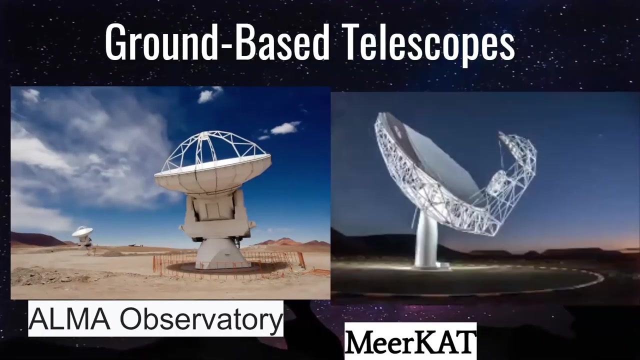 space, and typical example is the one we just um. so that is the answer c. now we will talk about the types of astronomical telescope observations. there are two main types of astronomical observation, and these are one ground-based telescopes, and these telescopes are telescope that observe the universe. 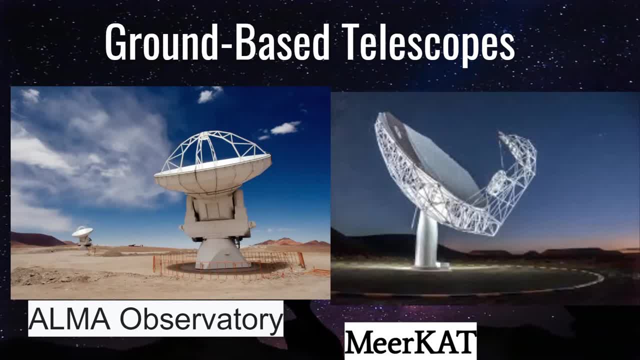 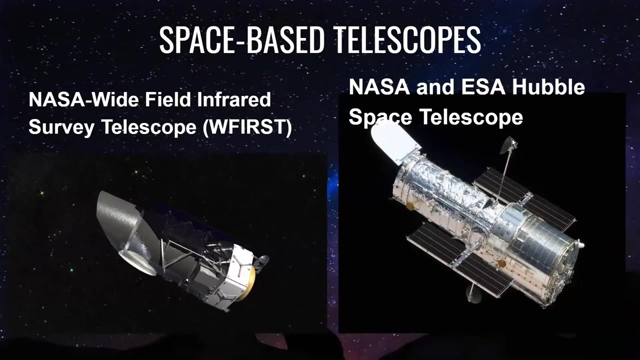 or observe the sky from ground. so typically they are built on ground and observe the sky, and example of such thirty- bald행, the alma observatory telescope and the meerkats, which is the precursor for the square kilometer array, located in south africa. and the second type are the space-based telescope. these are telescopes built in space to observe 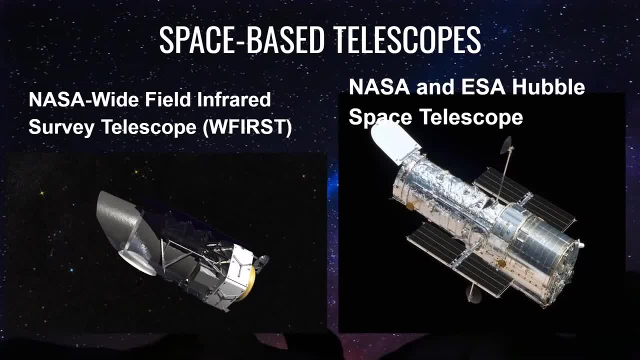 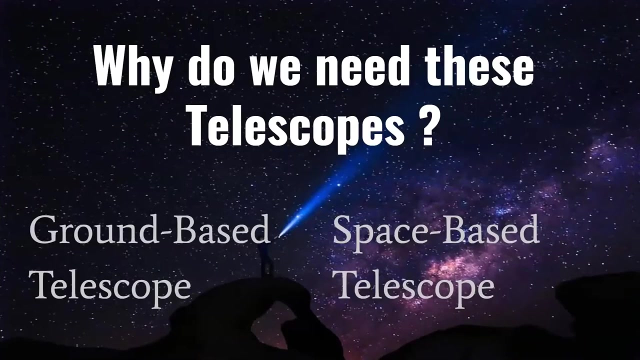 from space, or observe the ground or the earth from space, and typical example of such telescope is nasa whitefield infrared survey telescope, and another one is also the nasa and issa hubble space telescope. these are typical example of space based telescope. so again, why do we need these telescopes? either the ground-based telescope, 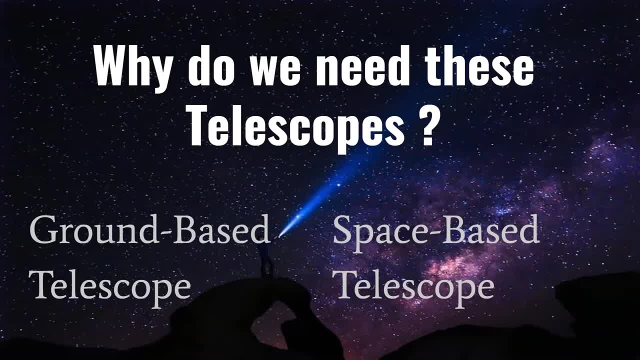 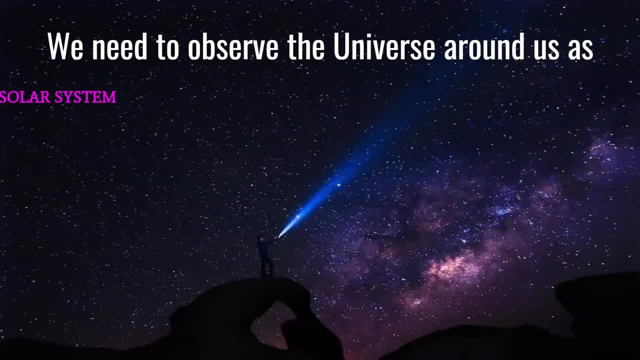 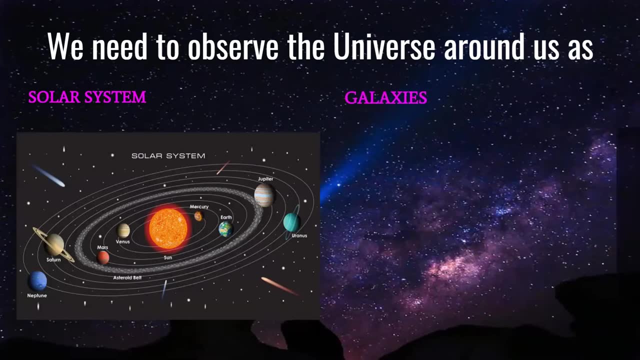 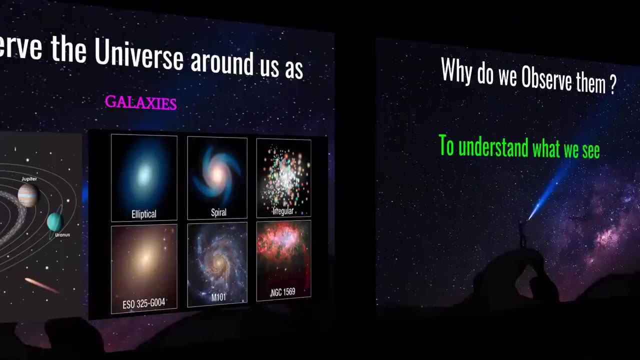 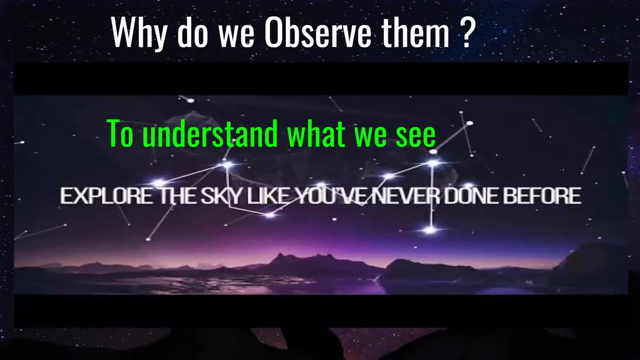 or the space-based telescope. we need them because we need to observe the universe around us as the solar system, as the galaxies. so why do we observe them, either in the form of the solar system or in form of galaxies? it is because we want to understand what we see very well and also do exploration, explore the sky. 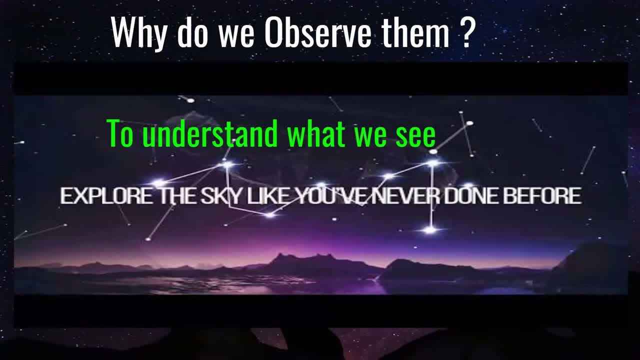 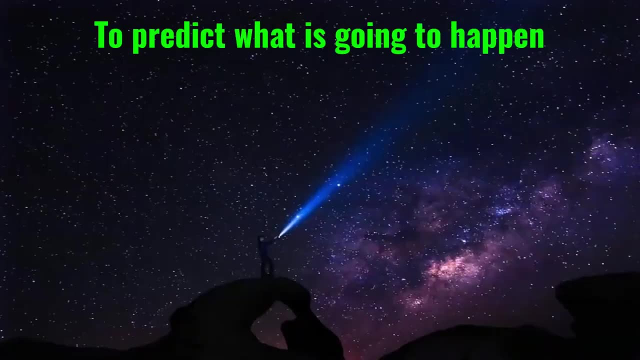 like we have never done before. these are some reasons why we have telescopes to observe the galaxies and observe their- the solar system, and another reason why we need them or we observe them is also to predict what is going to happen in form of asteroid and also in form of comets. 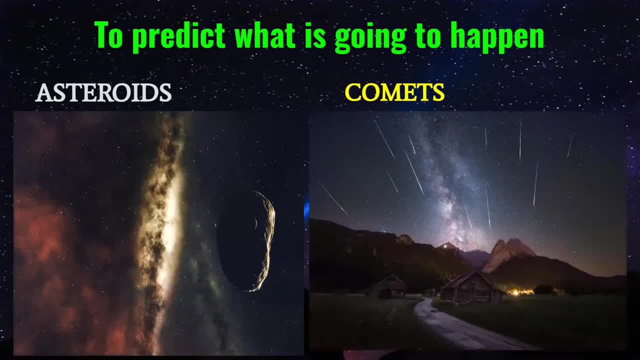 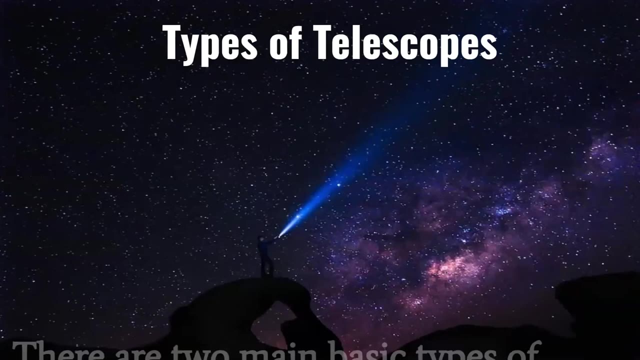 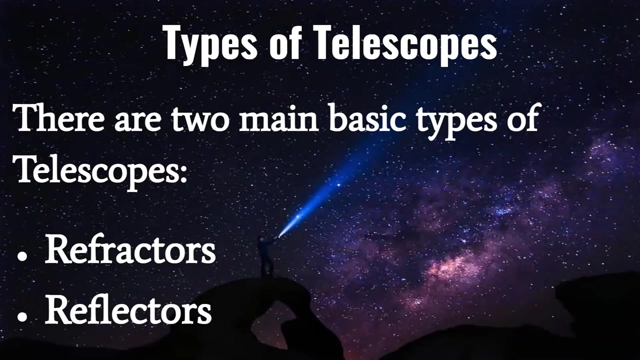 so observing them will give us a kind of understanding is going to happen ahead and if there's any thing we need to do or prepare, we must do now. talking about types of telescopes in terms of the construction, so we we learned about the the type of radio astronomical telescope observations. so both 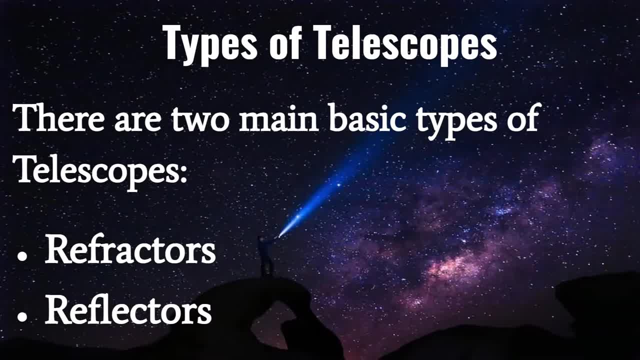 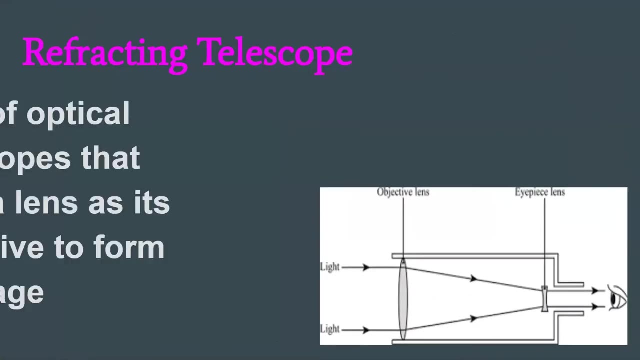 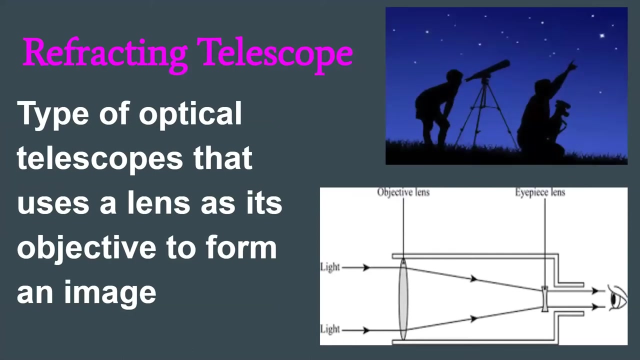 telescopes we heard about. we have two main basic types of them. one could be in form of refractors and other also be in reflectors. so refractors and reflectors refracting telescope- they are type of optical telescopes that uses a lens as each objective to form an image. 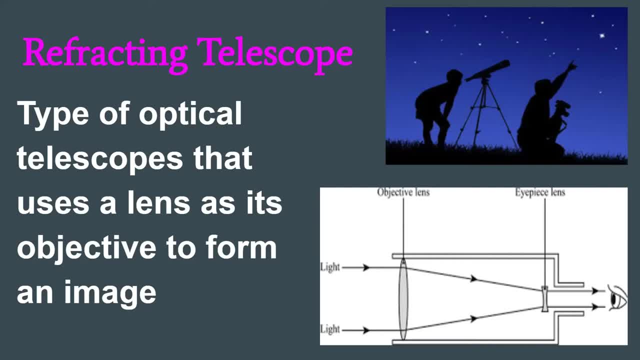 and the typical example is the one we are seeing in the picture and on the top and the block diagram or line diagram of that sat telescope is what we see with the eye piece or the lens. here we see the objective lens. this is the lens. so when a light fall on this, the light, 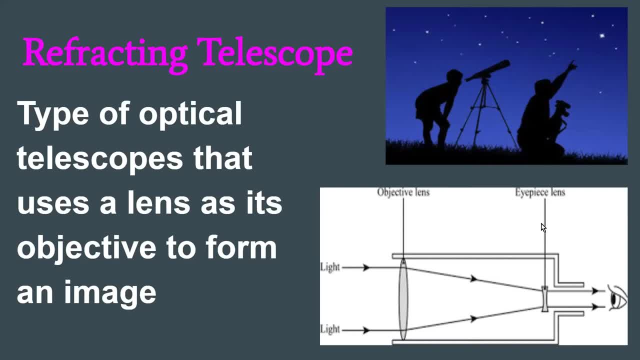 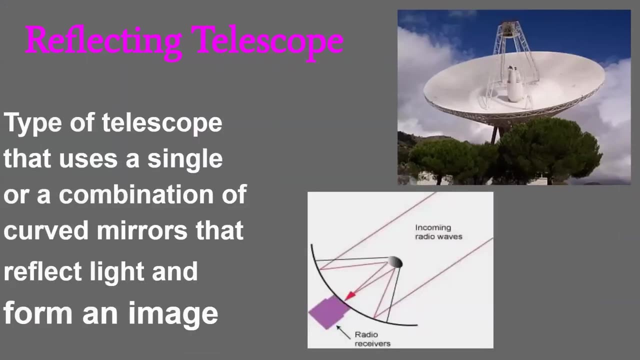 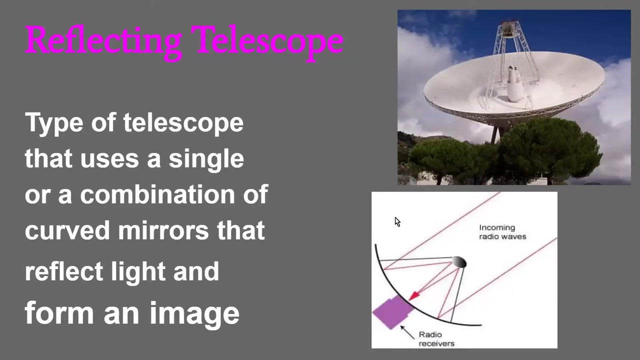 refracts to the eyepiece. so that is a typical example of um, the telescope we are seeing here and that's what we normally use here, and the other type, which is the reflecting type or telescope. they are also type of telescopes that uses a single or a combination of a curved mirrors. 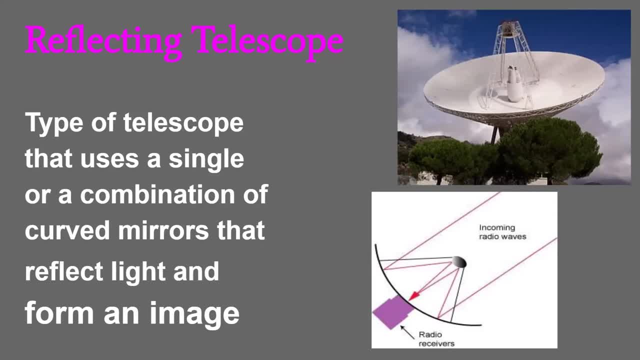 that reflect light and form an image, and a typical example of satellite scope is the one we see here, and the line diagram or block diagram of satellite scope is the one we see, the main 777. what about the other of some of the observable telescopes- orange, iron. 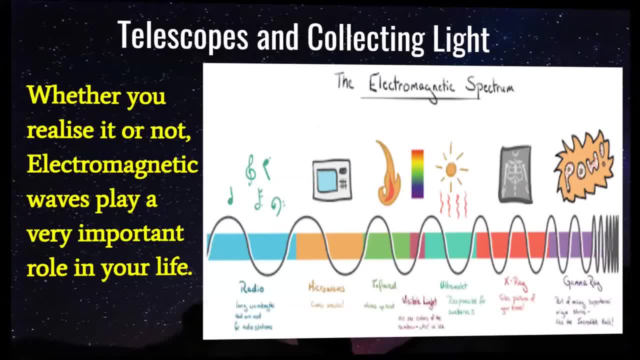 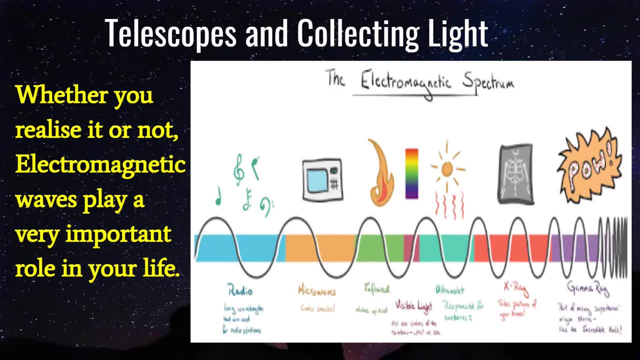 five, two, six, seven, eight and nine. seven, eight and nine and ten. two times 24. ions, Telescopes and collecting light. Telescopes and collecting light. So, whether someone realizes it or not, electromagnetic waves play a very important role in our lives. 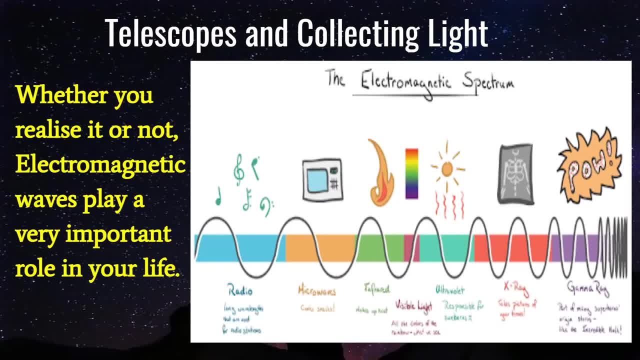 And these are the electromagnetic spectrum shown here. In our previous lessons about electromagnetic spectrum, we learned about the various electromagnetic spectrum, But here I'm there again and we are going to look at this electromagnetic wave and the type of telescope that observes each of them. 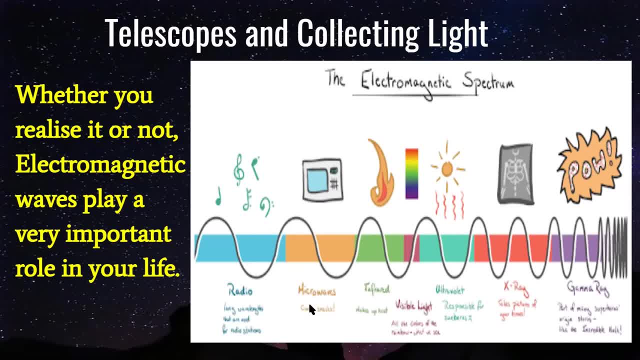 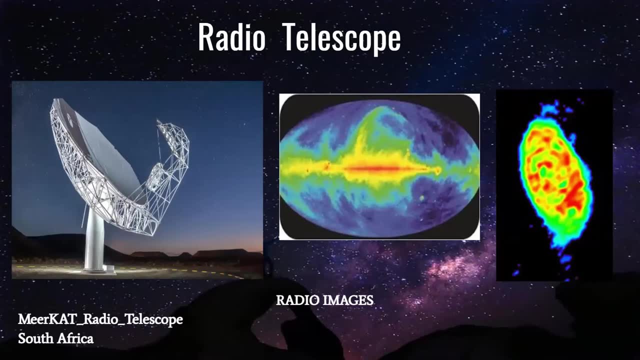 So we have radio here and we have microwave, we have infrared, we have ultraviolet and we have S-ray and gamma ray. The first one is radio telescope. So radio telescope are the telescope that collects electromagnetic waves, which is radio, or collects radio electromagnetic waves. 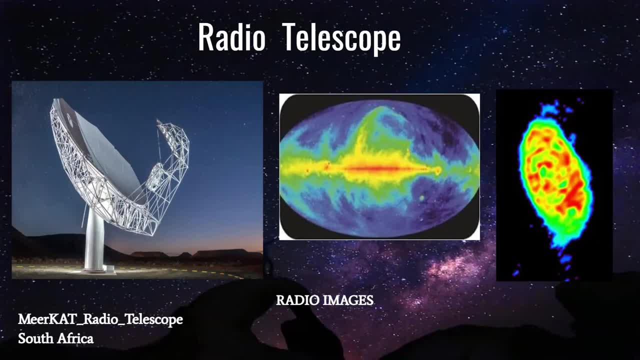 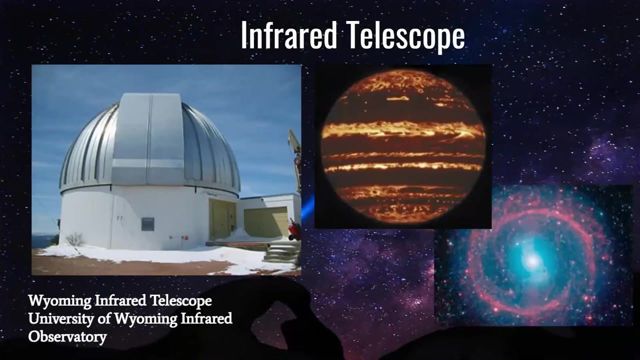 So this type of telescopes collect only radio waves, And typical example of image produced from such telescopes- radio telescopes- is the one we see here and another one here. The next one is infrared telescope. These telescopes are type of telescopes that collect only infrared waves. 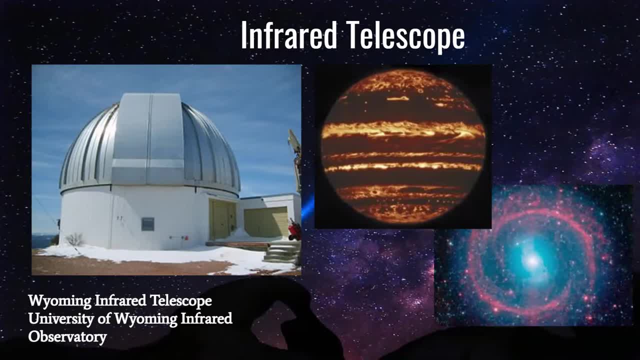 or infrared electromagnetic waves, And the typical example of such telescopes we have is Wyoming waves. Wyoming waves, Wyoming infrared telescope are from the investors of Wyoming infrared observatory, And the typical example of image produced from such telescope is the one we see beside. 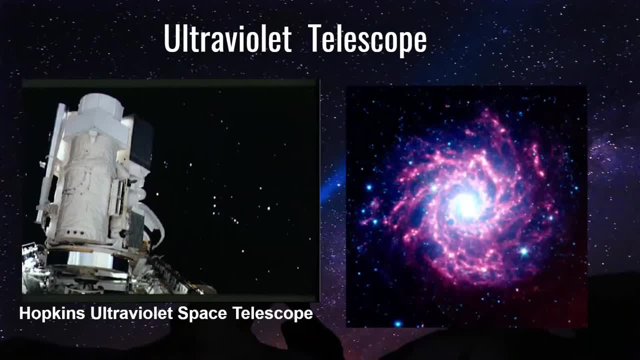 Another type of telescope, which is ultraviolet telescope, And this telescope collects only ultraviolet ultraviolet waves or ultraviolet electromagnetic waves. So these are telescope that detect only that electromagnetic wave, And a typical example of such telescope is a Hopkins ultraviolet space telescope. 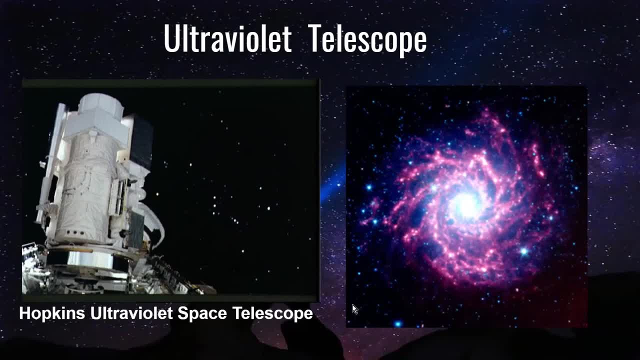 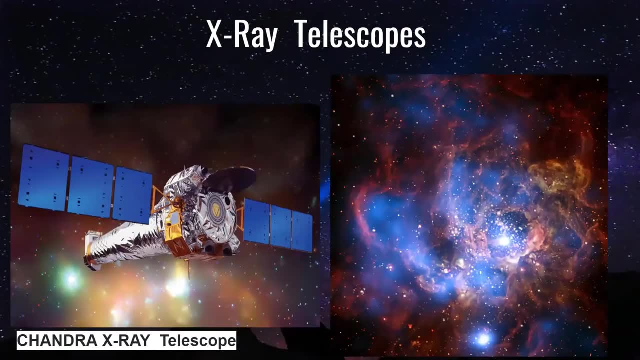 And a very beautiful picture beside it is an image produced from such telescopes. And then we have X-ray telescopes, And this X-ray telescope are type of telescopes that detect or collect only X-ray electromagnetic waves. X-ray electromagnetic waves. 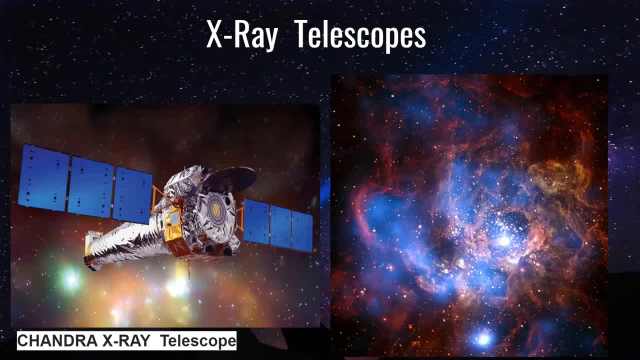 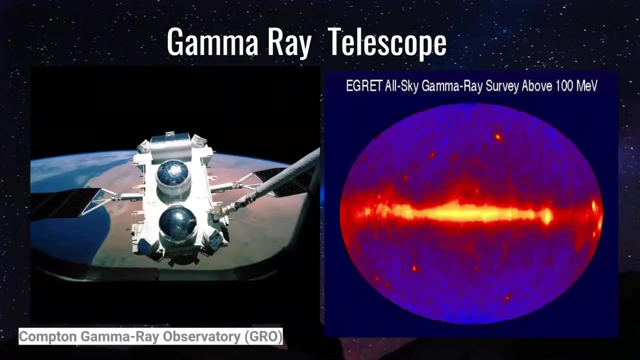 And a typical example of such telescope is Chandra X-ray telescope And beside this, a very, very beautiful image produced from this telescope. And then we have gamma ray telescopes And gamma ray telescope. Gamma ray telescope are type of telescopes that detect or collect gamma ray electromagnetic waves. 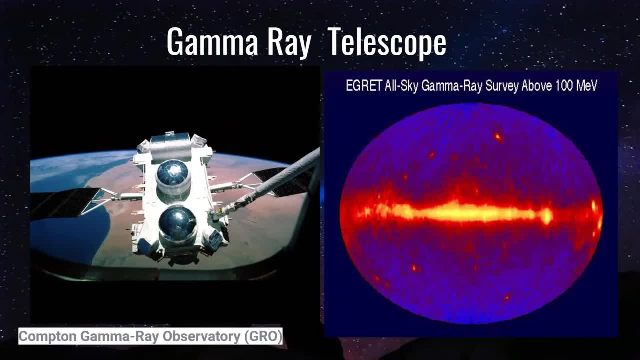 They are the only telescope that can detect or collect gamma ray electromagnetic waves, And a typical example of such telescope is a Campton gamma ray observatory. Campton gamma ray observatory And also we can see, uh, a very beautiful picture or image produced from such a telescope. 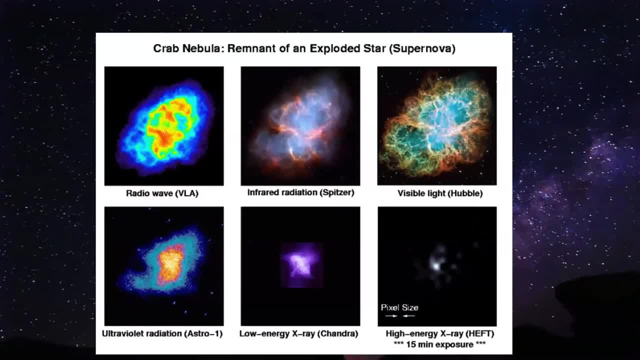 so, in conclusion, these are the various images produced from the various telescopes or various electromagnetic waves collected um by a different telescope. so a typical example of a particular source or particular um source, which is a crab nebula, uh, this is a super, super supernova, um star which has been collected uh using different telescopes. and these are: 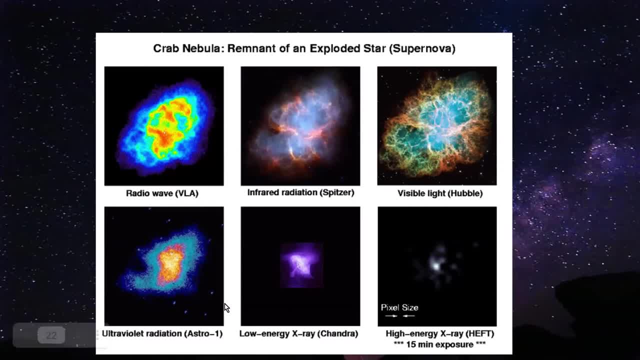 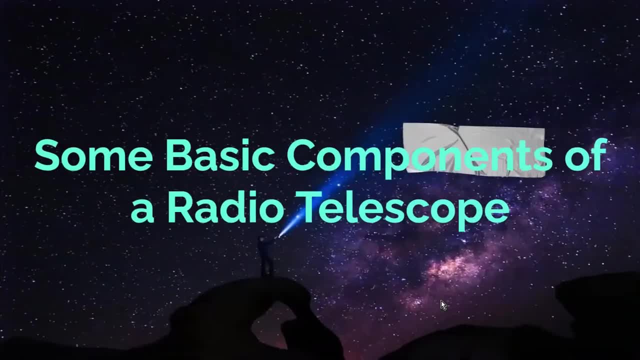 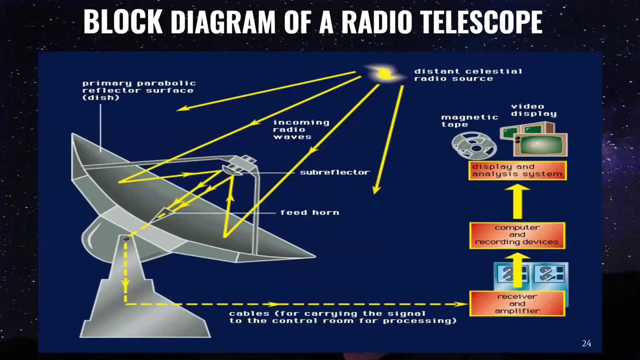 the images produced from the various uh telescopes from the same source of image now we now talk about some basic component of a radio telescope. focusing on basic component of a radio telescope, a typical diagram of a radio telescope shown here which we see: a telescope with um part. 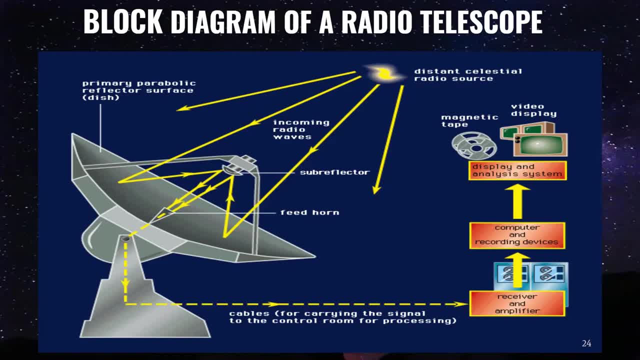 label and the first thing we see up. we see the dish which is a primary uh parabolic reflector surface or a dish, and we also see the sub reflector. we see the feed horn. we see also the incoming radio wave, which we learned about already radio wave. so these radio waves fall on the, the main reflector, and 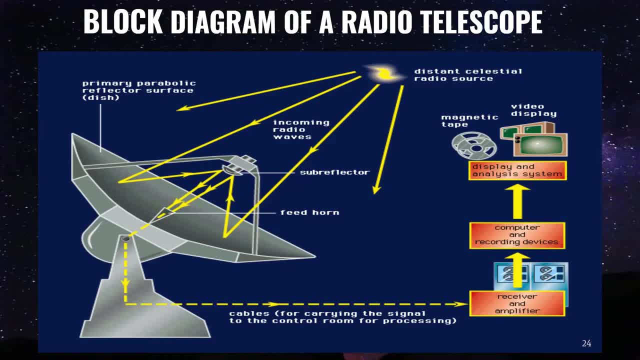 reflected back to the sub reflector, directed back to the feed horn and the processes happens into the computer or the receiver, the. the last or the final result is the beautiful image. so follow me and let's delve into this one by one and see the, the function of each component into detail. 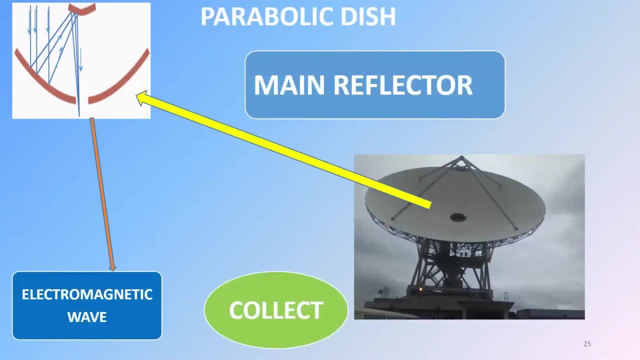 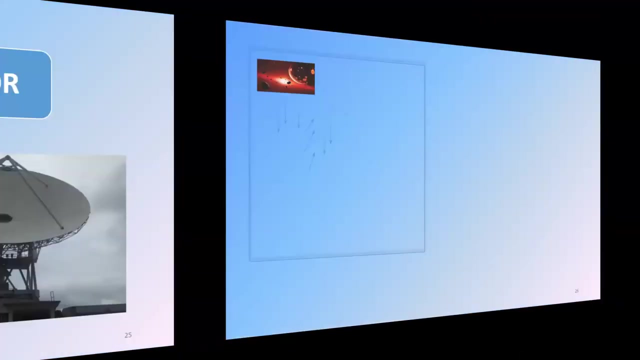 so we have the main dish, we have parabolic dish or parabolic reflector, also known Radio athletics provider. this main dish is also known as the main reflector. a function of this reflector is to collect electromagnetic width. the function of this parabolic dish, or the main reflector, is to collect electromagnetic width. 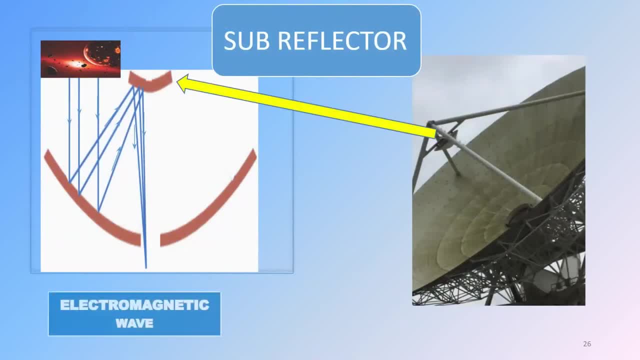 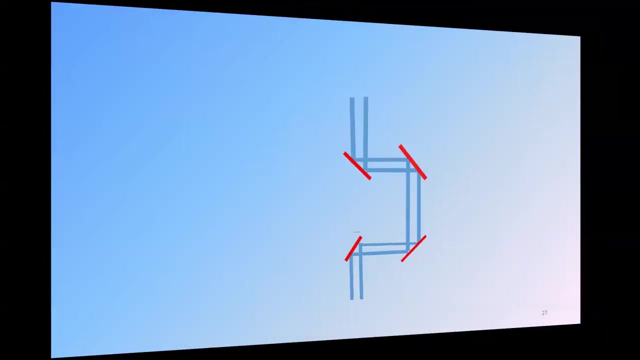 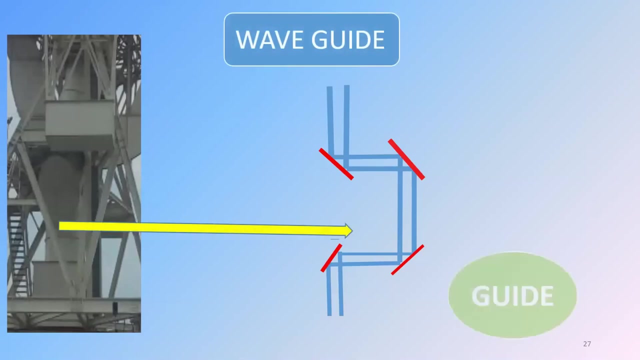 then we have the sub reflector. reflector is to direct the electromagnetic waves from the main reflector is to direct the electromagnetic wave reflected from the main reflector. now the next part or component is the waveguard, the waveguide. the main function of this waveguard is to guide the electromagnets, electromagnetic 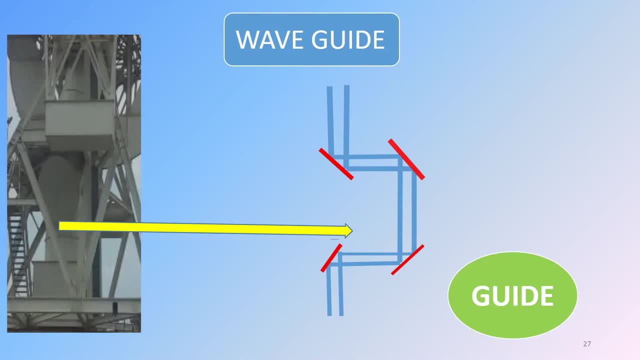 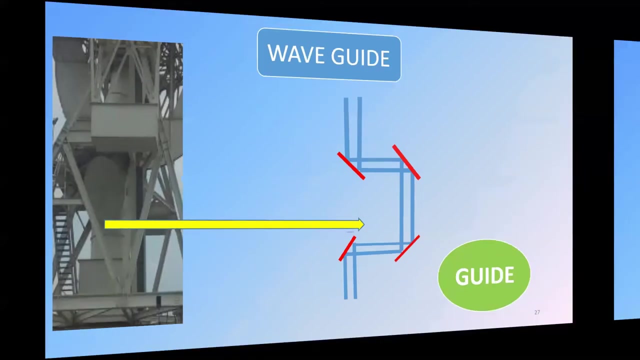 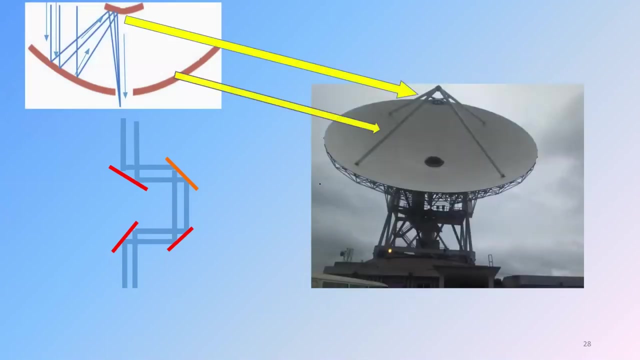 with, collected from the main reflector, directed by the sub reflector and guided by the wave guy. so the function of the waveguard is to guide the electromagnetic ways now. so we see here the labeling of all the tree that we had about and their functions. already the main 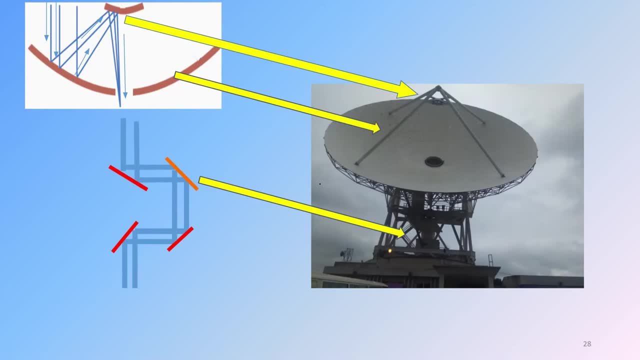 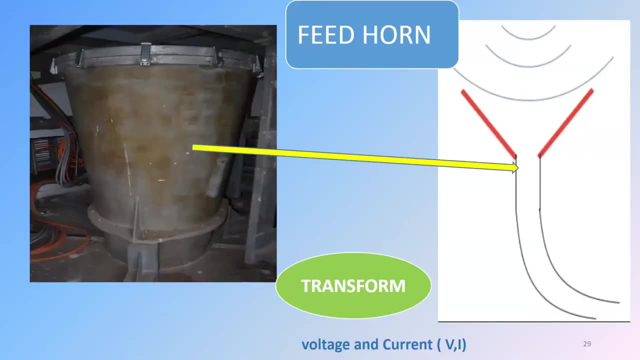 reflector, the sub reflector and the waveguard. now the next component is the feed horn. the feed horn, the feed horn. the function of the feed horn is to transform the electromagnetic waves collected from the feed horn. the feed horn is to transform the electromagnetic waves into boltages and go round. 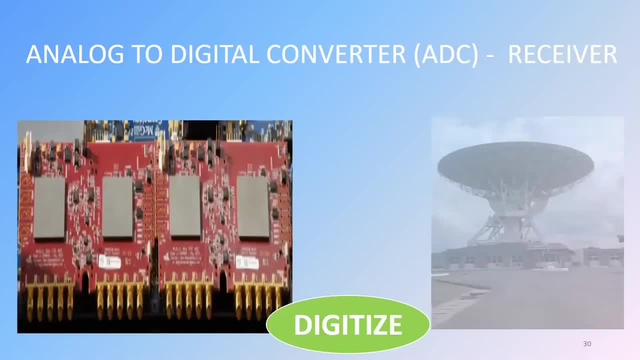 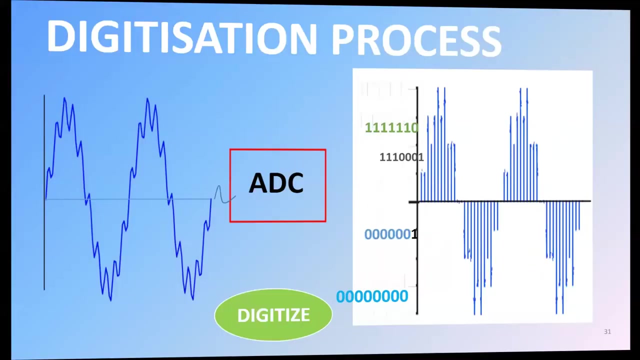 then the next part. the next part from the feed horn is to either to lower lowfoil position, position position position called as receiver. the function of this receiver is to digitize. digitize the voltages and the current collected from the feed horn, from the adc part. then we come to the digitization process. 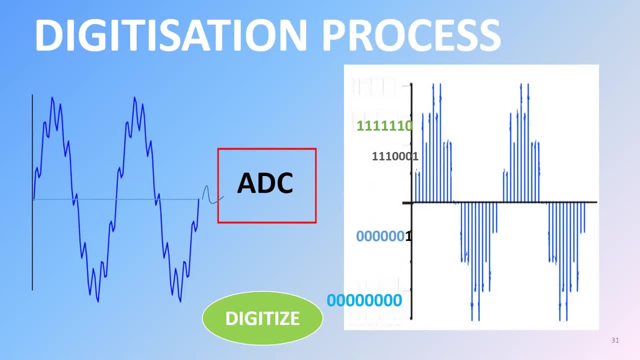 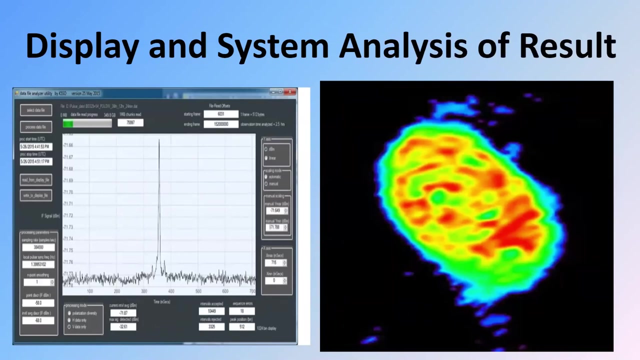 or digitization process. so this is where, from the adc part, which digitize the, the, the, the voltage and the current received in this form, digitized into a digital signal where we had our receiver, or the computer can now will recognize as zeros and ones, and then the next thing we see, or the next part, which is the display and system analysis of. 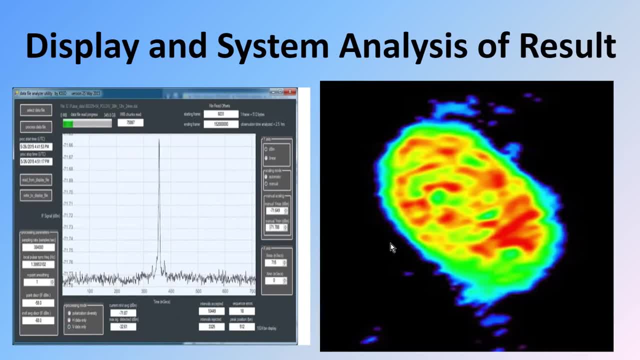 results. so what we see next, uh, is the, the display of the analysis of the results after the digitization, where our computer can read or recognize the zeros and ones in the digitization form. so this is what we see, then. the next thing is to see our beautiful image of such a source. 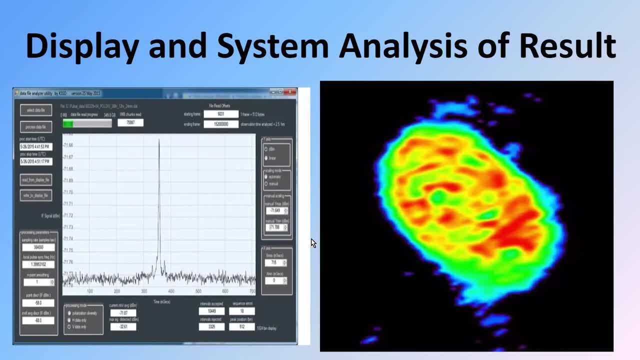 or celestial source that we are looking at. we focus our telescope or the main reflector. so meaning that the main reflector is looking towards or collecting electromagnetic waves from this source. so this is what our um, a telescope or main reflector, uh is looking at. so this is a beautiful result. 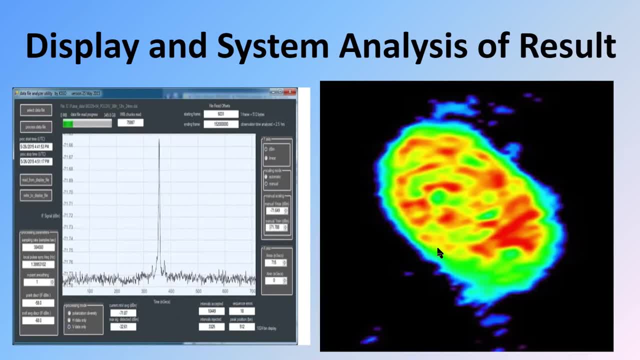 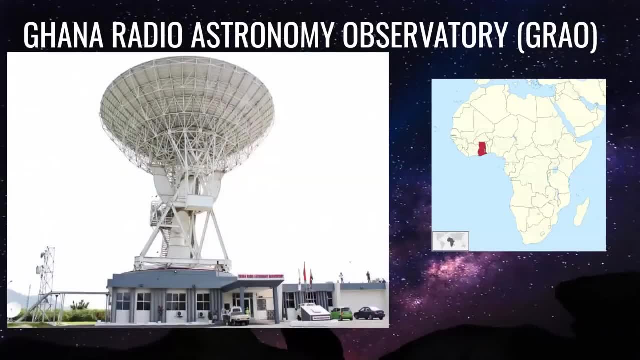 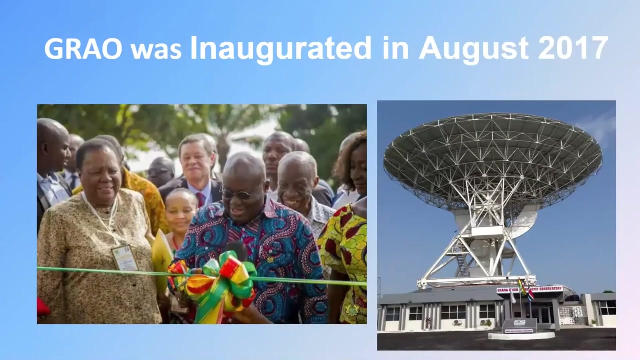 that we have here. that is how the radio astronomy telescope function. now we'll talk about the ghana radio astronomy observatory. crowd, located in ghana and the capital city, accra, and in kutusi, and that is ghana radio astronomy observatory. so grow, or ghana radio astronomy observatory, was 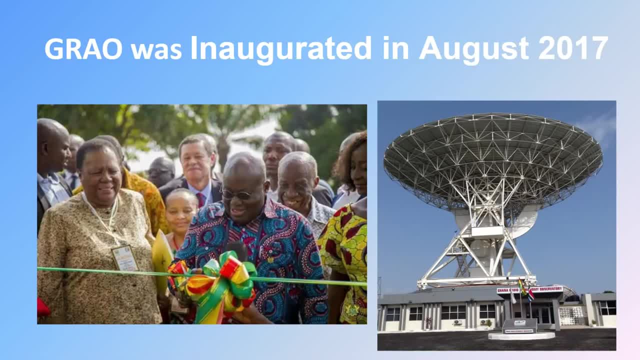 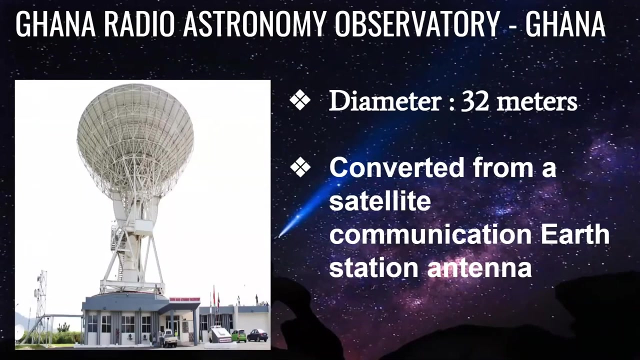 inaugurated in august 2017- 2017- by the president of republic of ghana, assisted by the then science and technology minister of south africa. ghana radio astrono observatory um ghana is a 32 meters dish. so when you say the dish as the main reflector, we learn about that- the size of it. 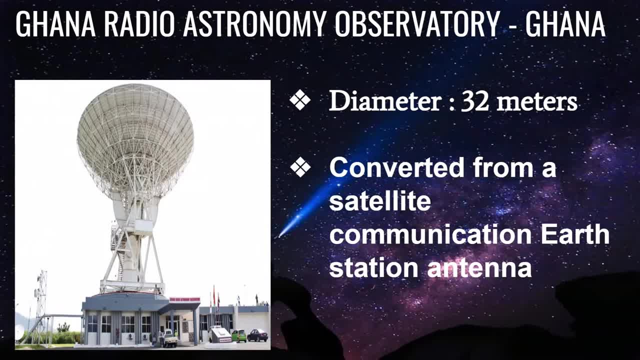 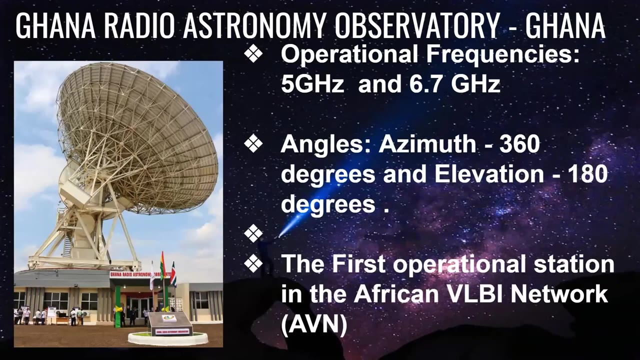 the size of it is about 32 meters. so this was formerly, um, a satellite, a communication earth station antenna, and it was then now converted into a radio astronomy instrument or telescope. so a few more about ghana radio astronaut observatory. um, it operates, uh, at a frequency of 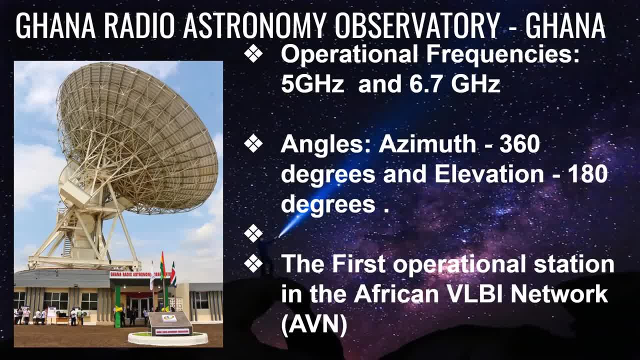 five gigahertz and to 6.7 gigahertz. and another important thing we also have to look at and we talk about the angles of this telescope. when we talk about azimuth, it tends, uh, clockwise 360 degrees. that is the azimuth elevation. that is azimuth elevation it takes. 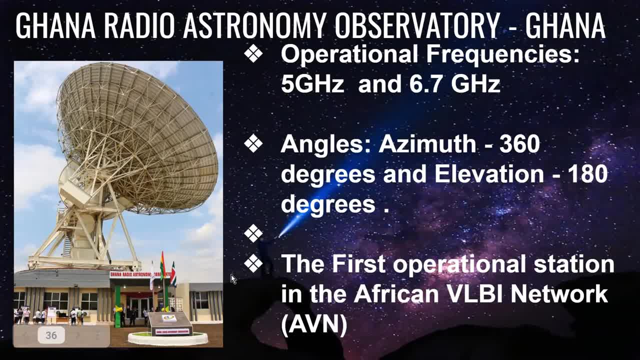 or it retains on each angle clockwise, 360 degrees. that is operating angle and we have elevation of 180, so it sees the horizon from zero raise up to another side of it, so up to 180. that is the elevation from up of, from down, up down. it also has the operated anger of 180 degrees and it's also very important to